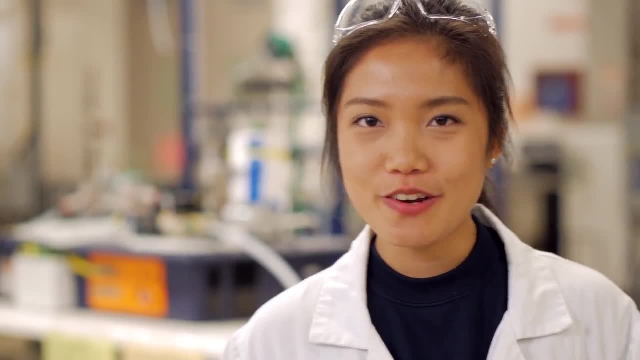 I'm also the Co-President of CHEMICAL and BIOLOGICAL ENGINEERING. I'm also the Co-President of CHEMICAL AND BIOLOGICAL ENGINEERING. I'm also the Co-President of CHEMICAL and BIOLOGICAL engineering undergraduates. this year There's a lot of activities that we put. 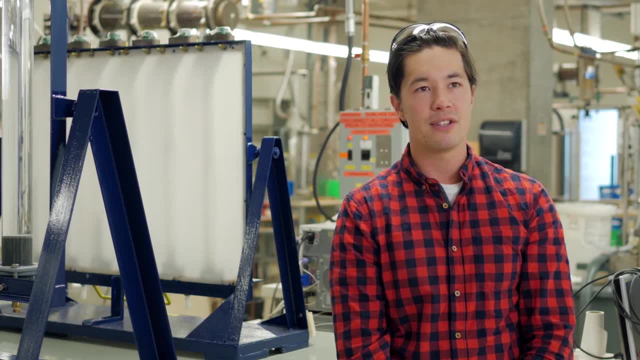 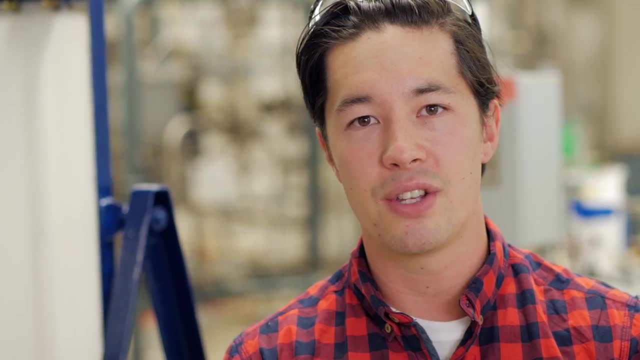 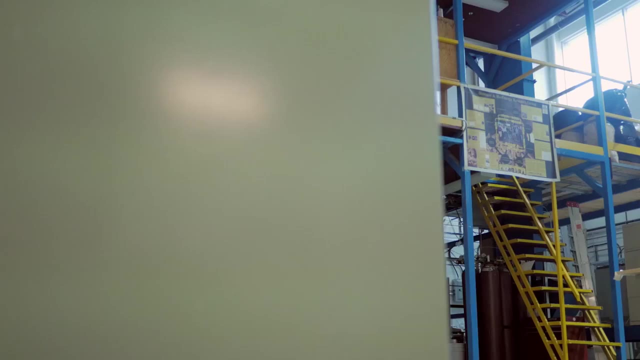 on as a student council. You're spending a lot of your days with the people that you're graduating, going to classes with and eventually going out after classes as well. It's really a family. by the time you're at your fourth year, Our laboratories provide students excellent training. You are exposed to 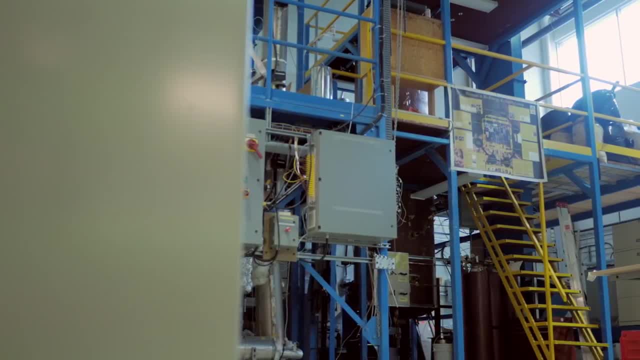 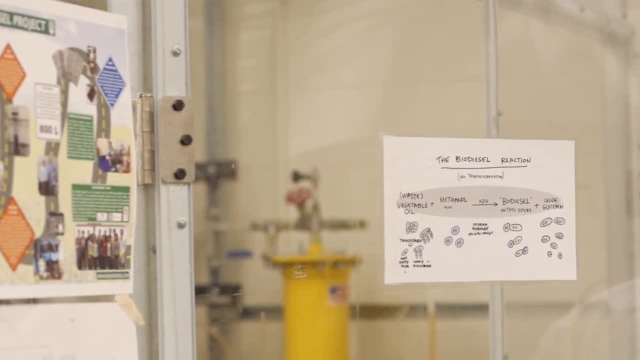 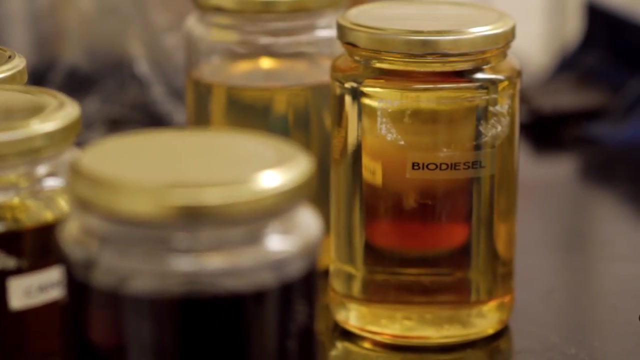 miniaturized industrial processes, essentially smaller versions of the real processes that you see in the industry. Right now we're in the biodiesel lab, and in this lab we create biodiesel, so a more environmentally and socially responsible way of getting energy. What we're seeing is that environmental 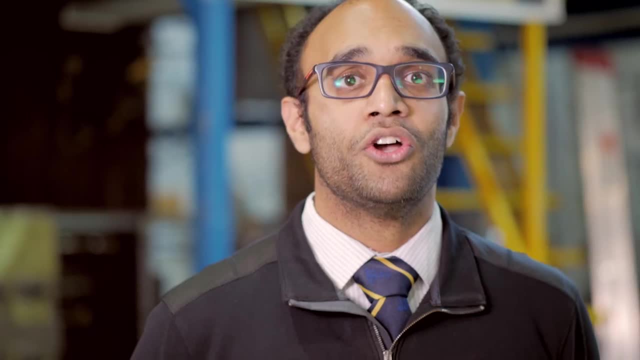 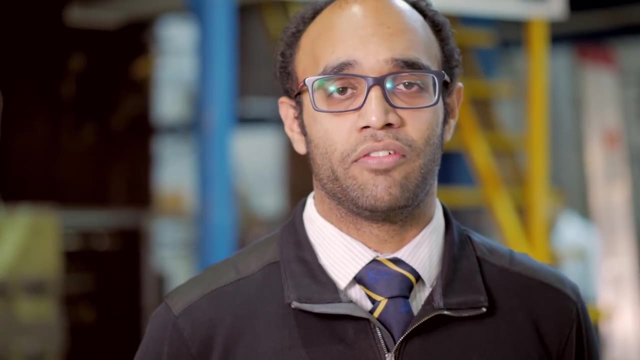 engineering has essentially fused into chemical engineering. So all the processes, all the engineering that we do, environmental responsibility is the number one design rule that we have to follow. For example, chemical and biological engineer work in the chemical engineering field is a very important. 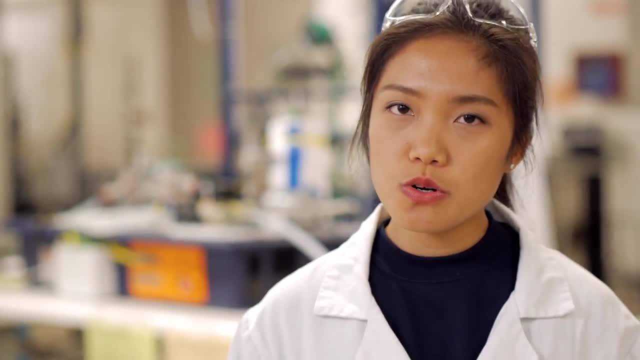 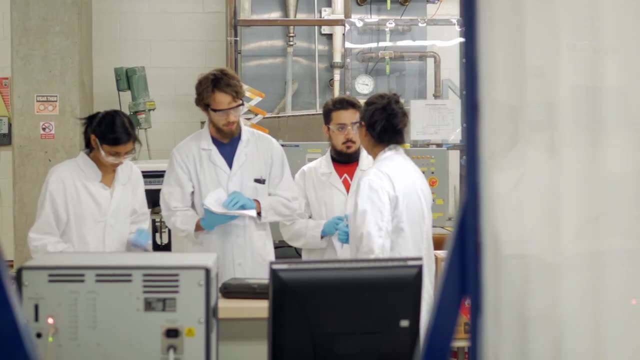 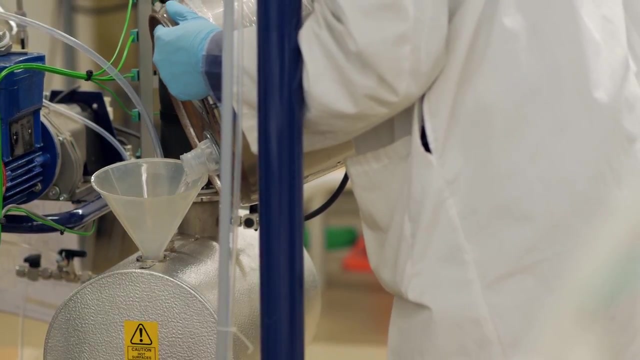 part of our research. We take courses in water treatment plants. we take courses about air pollution control. we learn how to make use of alternative energies and how to improve these processes. The research ecosystem at UBC is amongst the very best in the world. What ends up happening to a lot of our undergraduate? 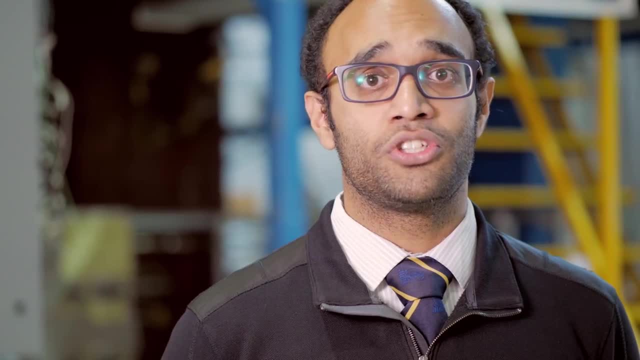 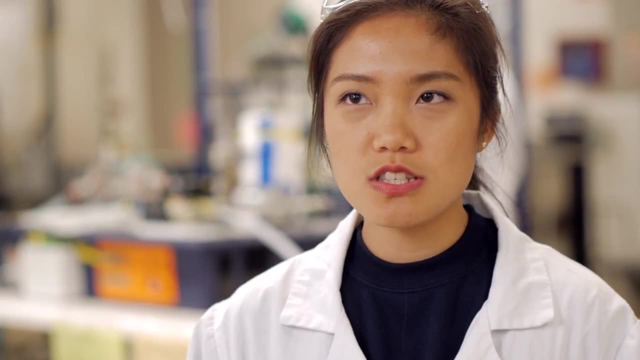 students after they've been exposed to this rich collection of research topics is that a lot of them eventually decide to pursue medical school or graduate school in some of the very best universities in the world. Biological engineering just opens so many doors. It's very versatile. so if you look around you, 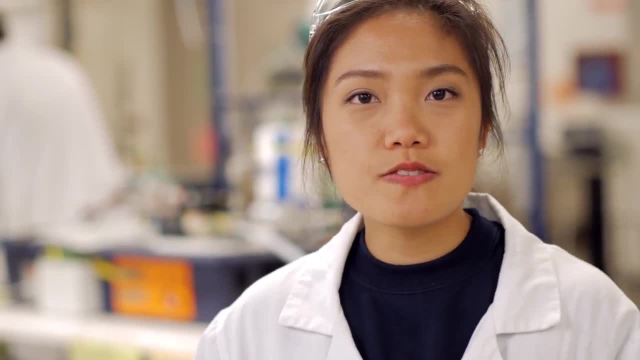 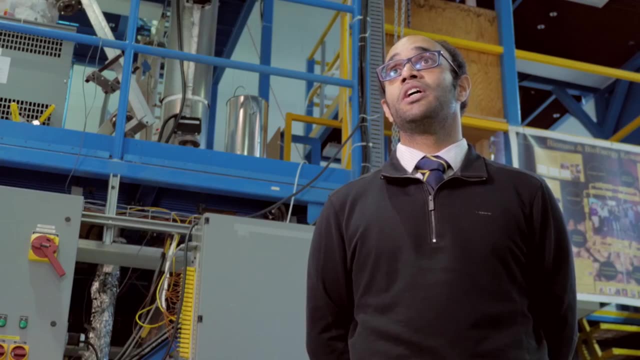 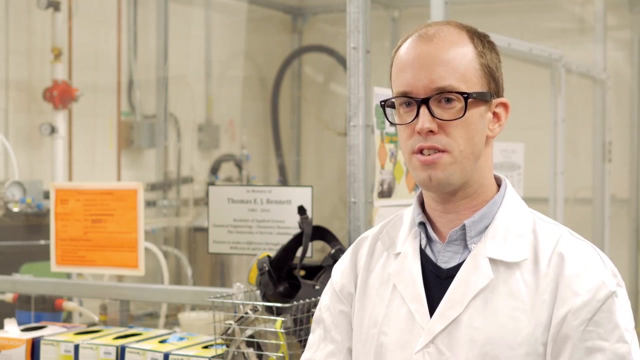 anything that you see, if it involves any process in making that product, you can work in that industry. It is a truly transformative experience for our students because it opens up career options and their horizons in ways they had never even thought about before. I think if you're interested in an 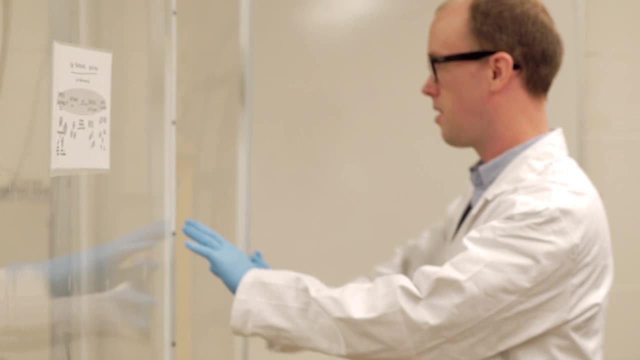 exciting and challenging career in production and also sustainable engineering, then this might be the place for you. I think it's a great field for you.